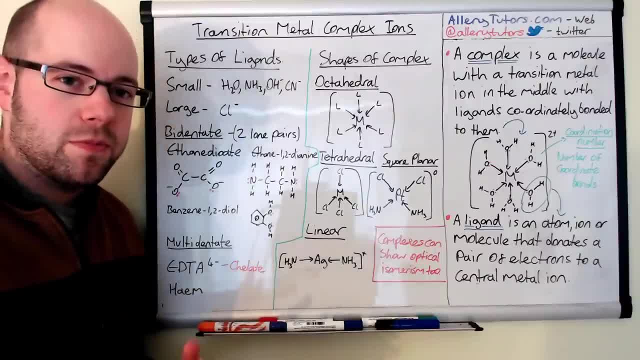 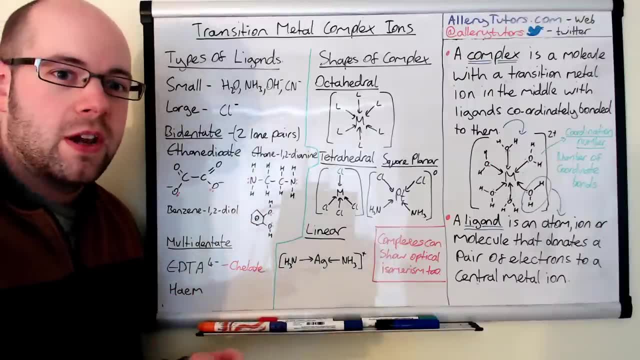 the co-ordination number. The co-ordination number tells us the number of coordinate bonds that surround our metal ion in the middle. So you've got to be careful not to confuse this with the number of ligands that surround the metal ion as well, because we'll come on to that. 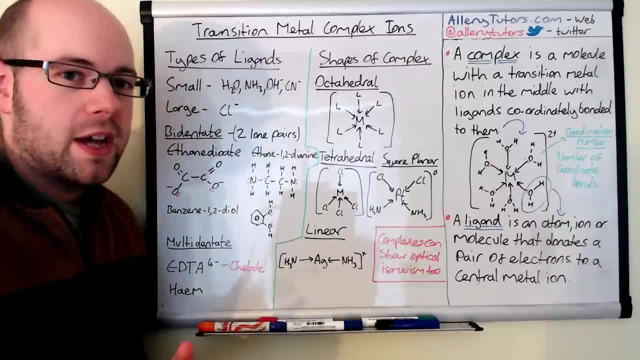 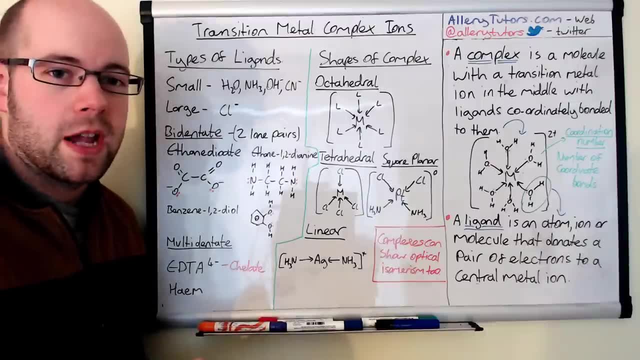 in a minute, where some ligands can actually bond twice, and so the co-ordination number is the number of coordinate bonds that is surrounding the metal ion. So you've got to remember that. Okay, so we're just going to look at some of the types of ligands as well. You can 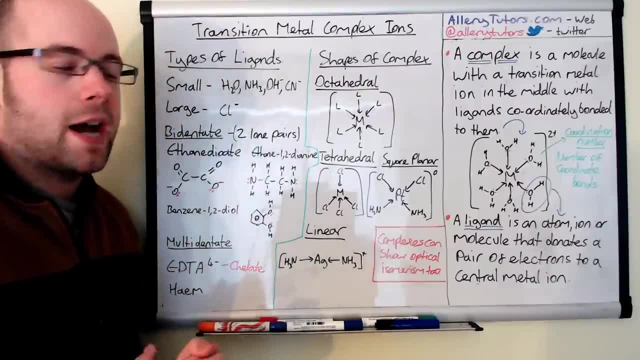 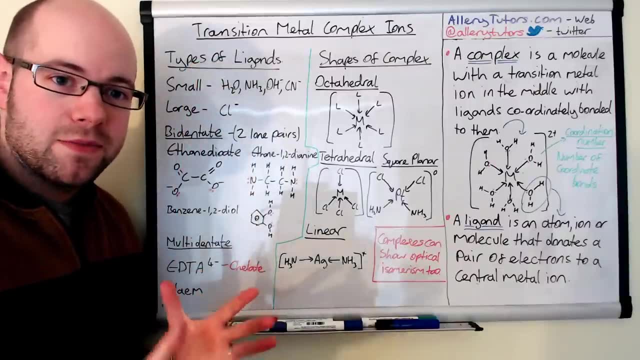 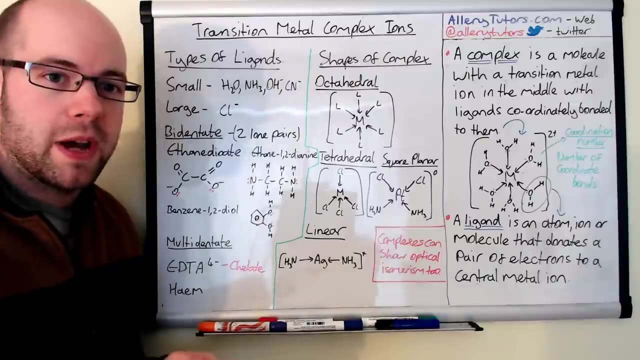 see here that I've listed a few different types and we have something called monodentate ligands. and monodentate ligands are, like I say, atoms, molecules or ions which effectively only have one lone pair. well, they only donate one lone pair to the metal ion in the middle. Some of them might 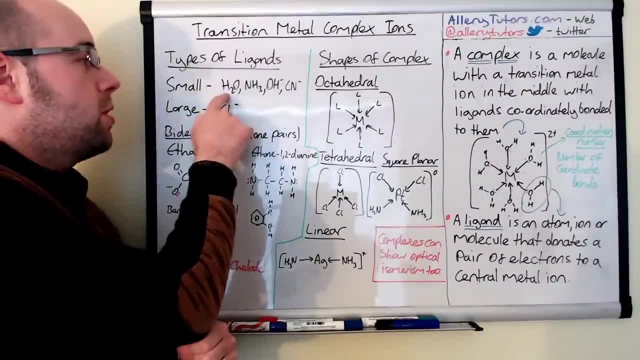 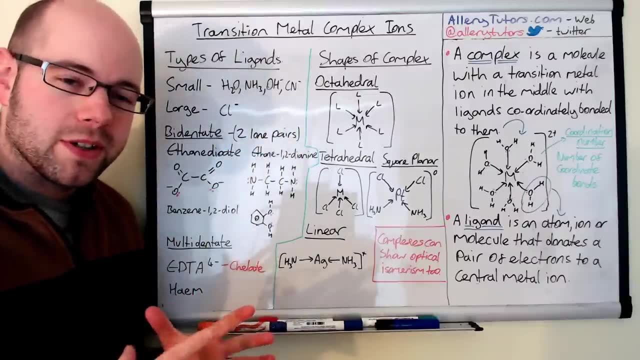 be more than one lone pair. So, for example, we're going to look at water, ammonia, hydroxide, cyanide, and these are all classed as small ligands, and this is important because small ligands, you can fit more of them around the transition metal line in the middle, whereas opposed to large, 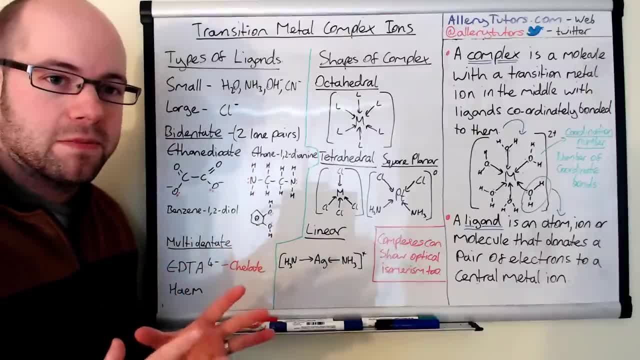 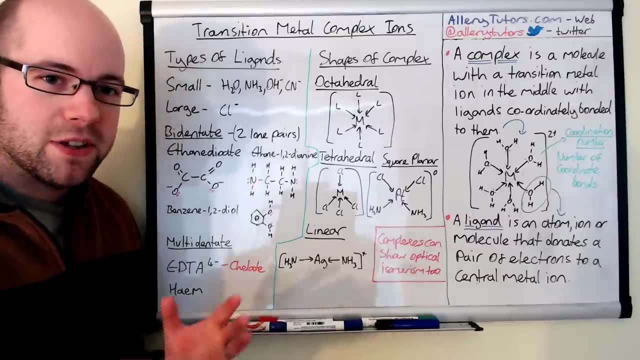 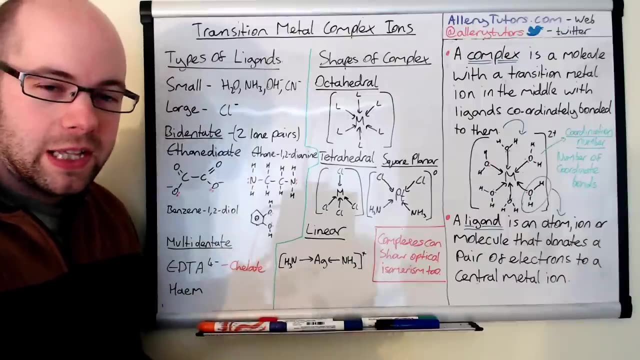 ligands like chloride ions, which are obviously a bigger atom. in general you can't fit as many of them around the metal line, so it's a little bit like, I suppose, like pigs around a trough. So you might have your ligands being like pigs and the meth line is like the trough. Some pigs, little pigs. you can fit six of them. 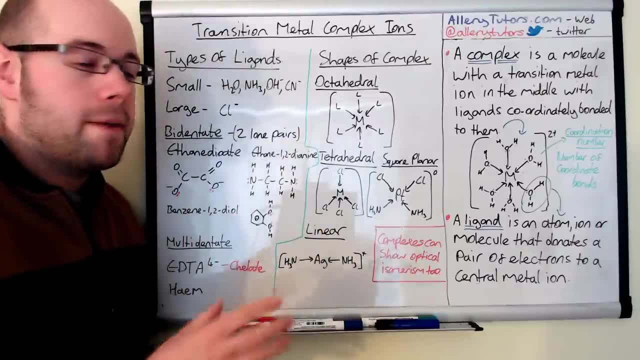 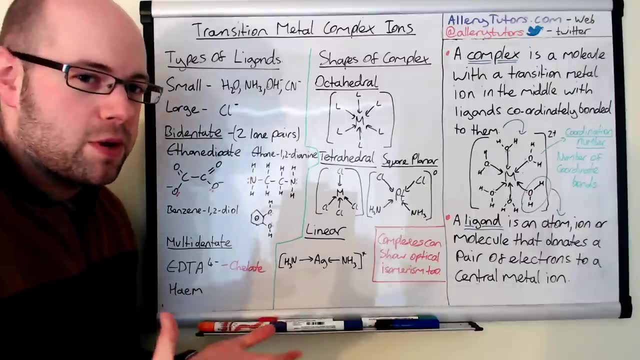 effectively around the meth line, which we'll look at in a minute. Whereas the larger ligands- these are like the fatter pigs: you can't fit as many of them- pigs- around the trough, So you might say you'll be only able to fit four of them around the trough, whereas the smaller ones you can fit. 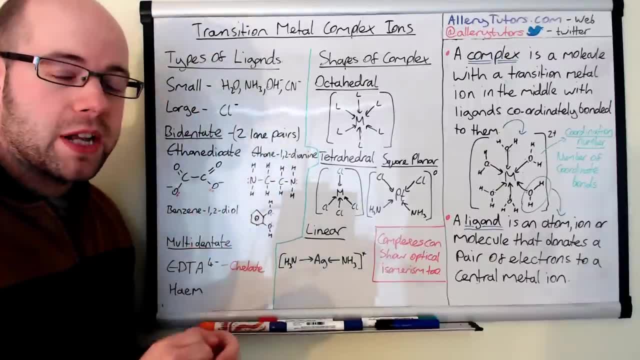 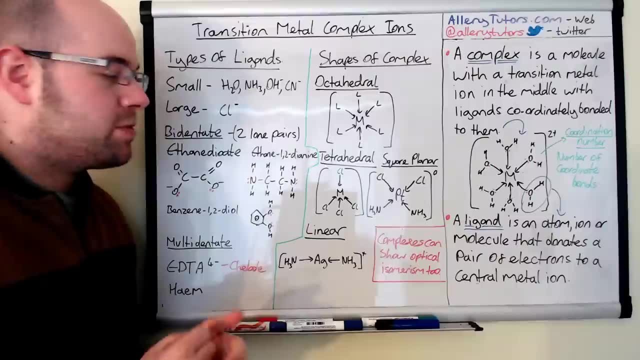 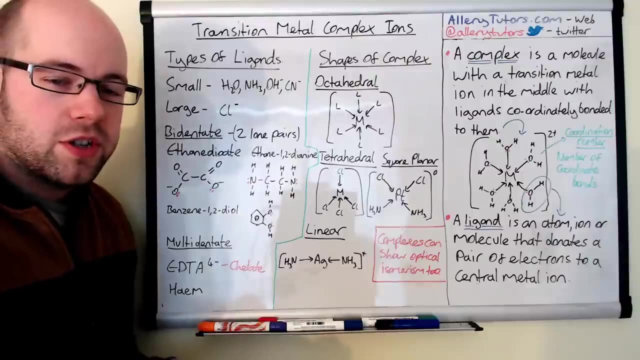 six of them. So these are classed as monodentate ligands because they only donate one lone pair to the meth line in the middle. Okay, sometimes we can have bidentate ligands and this means that they can donate two lone pairs of electrons to a metal ion in the middle. So, for example, 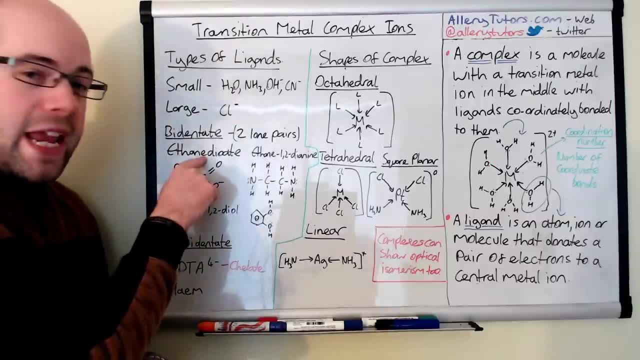 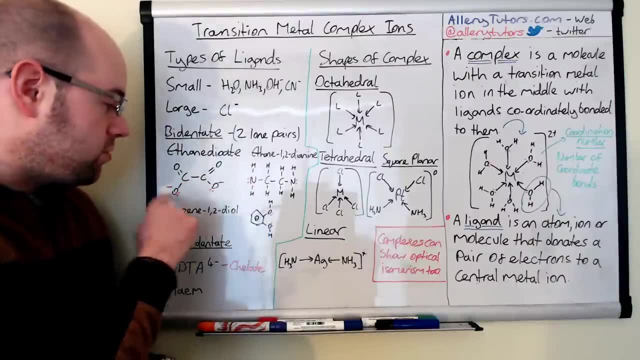 we've got something called ethane diuret. Make sure it's got the E in there as well. that's really important And you can see it's basically just a dicarboxylic acid. It's got hydrogens missing from it in the middle And where the hydrogen would have been on the carboxylic. 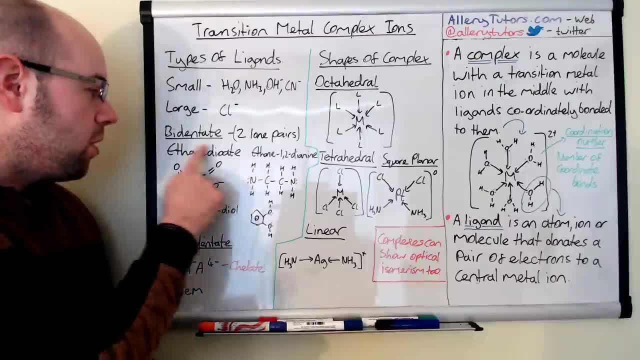 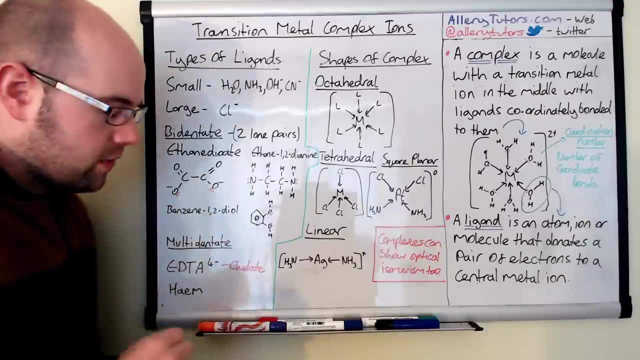 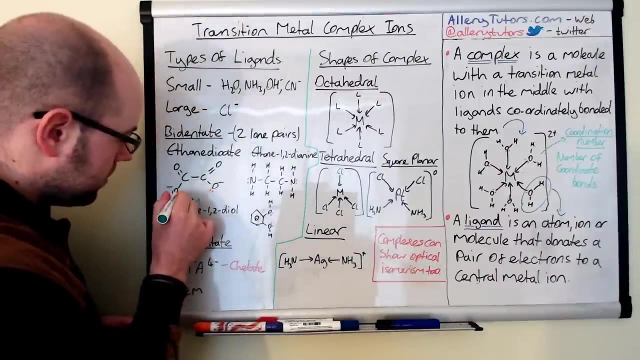 acid. we have a negative charge on both ions. So overall this ligand is two minus charge And we have lone pairs on the oxygens here. And effectively how this would work is you would have- and I'll do this in green- is you'd effectively have a metal in the middle and this can bond twice to the 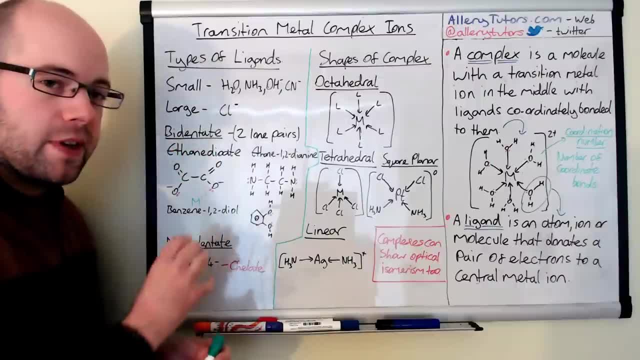 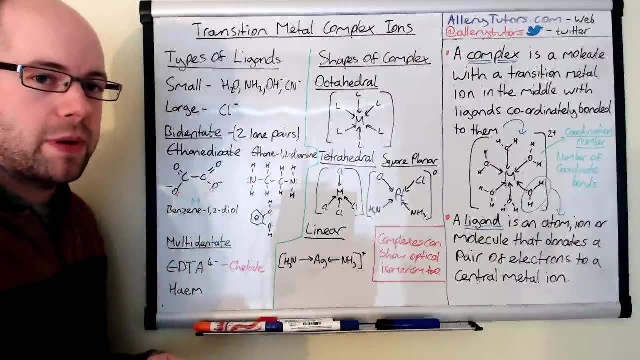 metal. So the one ligand bonding twice. So this is effectively classed as a large ligand, obviously no surprise. And hence you can't fit many of these types of ligands around a central metal ion. But again, we'll have a look at that as well when we look at the complexes. 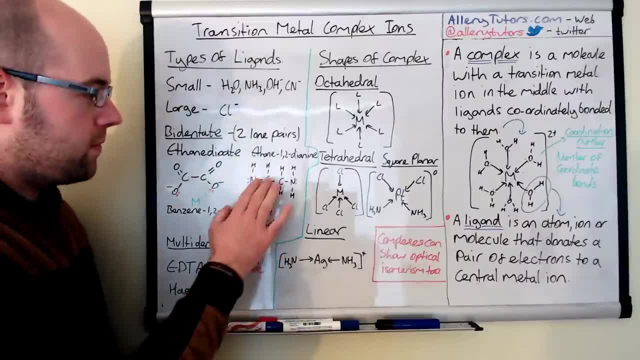 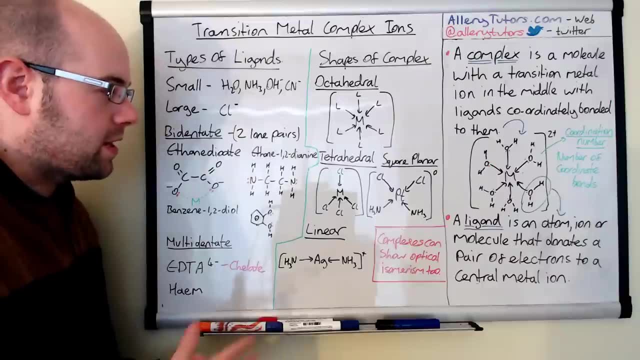 Okay, here's another one: ethane 1,2-diamine. Again, we've got ethane in the middle and amine grouped either side, And amine is NH2.. We've got two of them either side there Again. 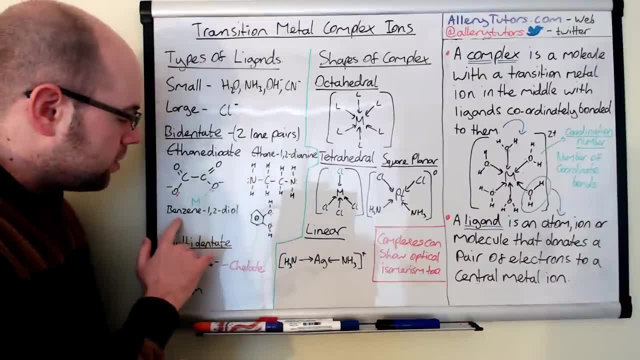 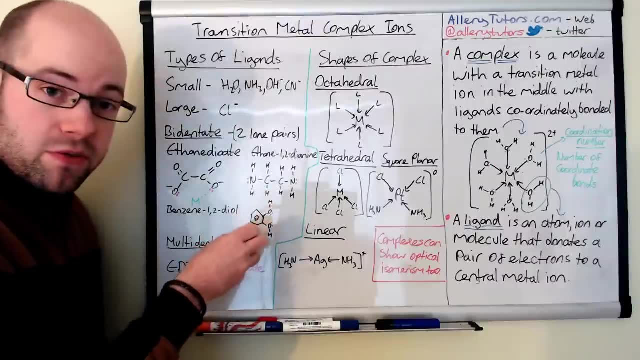 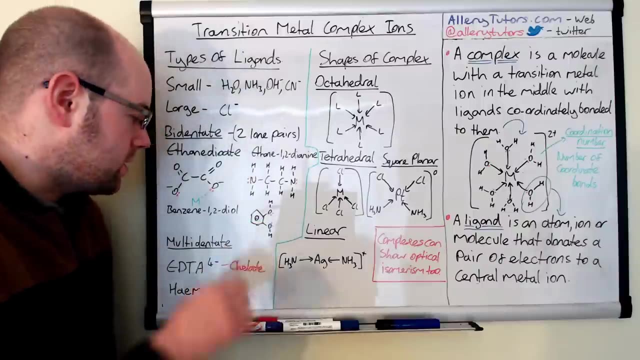 with the lone pairs on the side, so this can bond twice, And another one which is benzene 1,2-diol. So again it's just a benzene group with two alcohol groups coming off it. We have a lone pair of electrons on each oxygen And again, a bit like the ethane diorates it can. 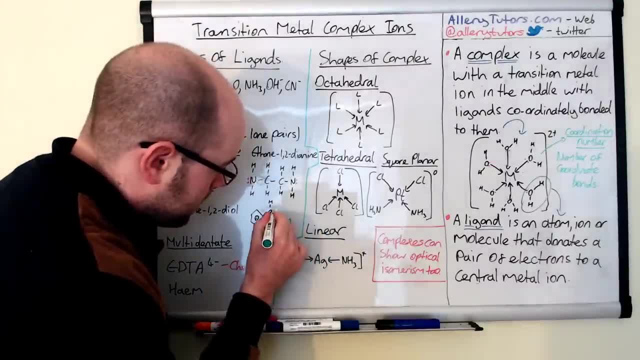 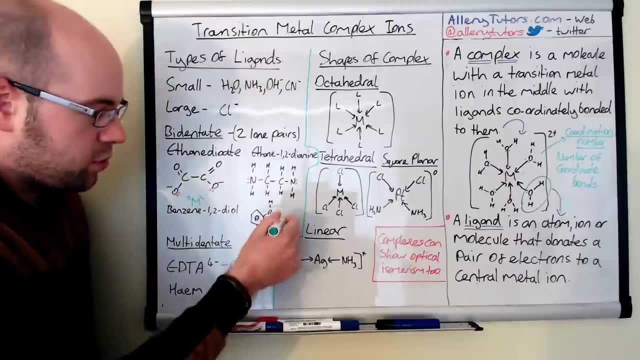 bond twice. So if I put my metal there and you can see, so I put my arrows just to show that they're coming in and bond, There you go And it can bond twice to the metal ion. Again, these are large ligands. You can't have many of these around a metal ion. They're a lot larger. 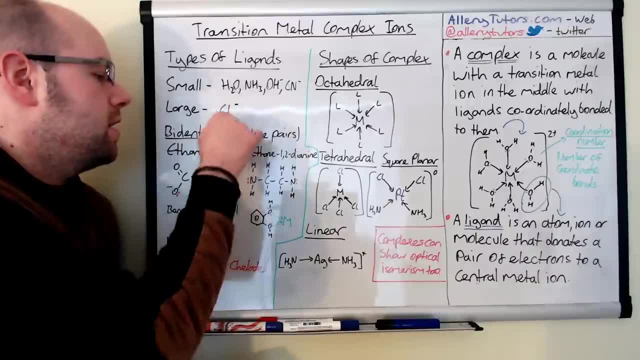 than even the large monodentate or unidentate ligand on the top there. Some ligands are even bigger And we've got a lot of these ligands here. So again, these are large ligands And again you've got ones here. You don't need to know the structure of these, thankfully. 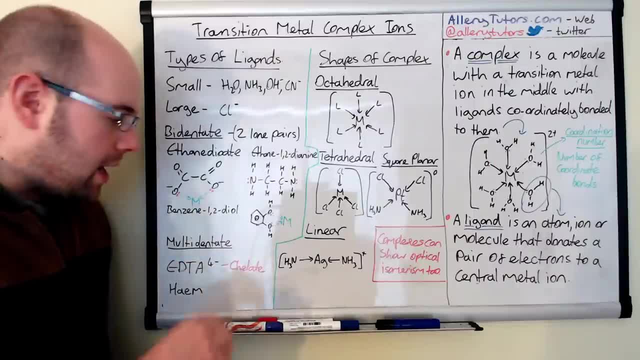 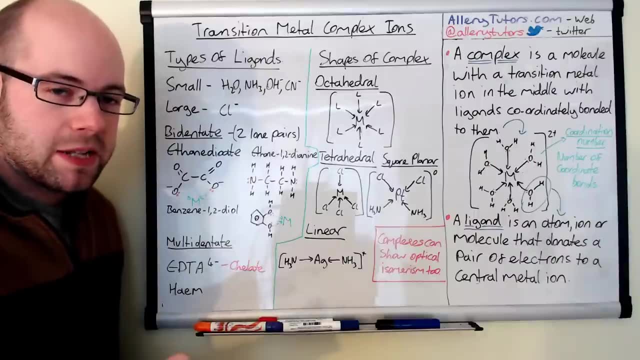 because they're really complex. But this one here is EDTA. It's really good. It's really good at removing potentially toxic metals from the blood And it can be given as a medicine to remove that. So, for example, you've got lead poisoning. It can bind with the lead really well And we call that. 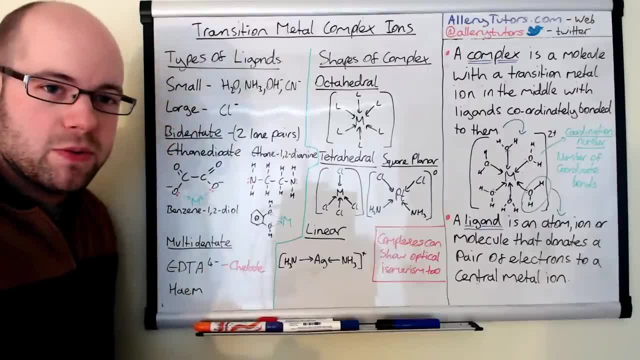 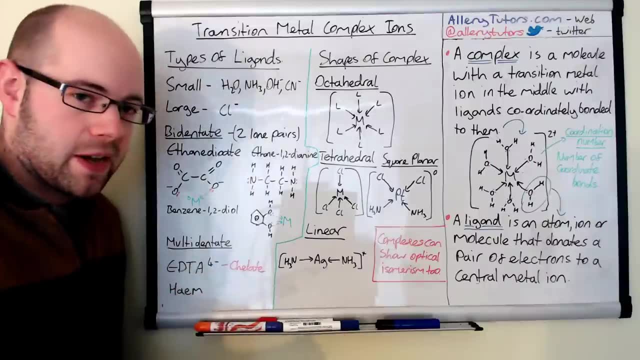 a chelate And effectively it comes from the Greek, which means claw, a bit like a crab's claw, And multidentate ligands have a chelation effect, So they effectively bind themselves multiple times around the metal ion in the middle and effectively sometimes even. 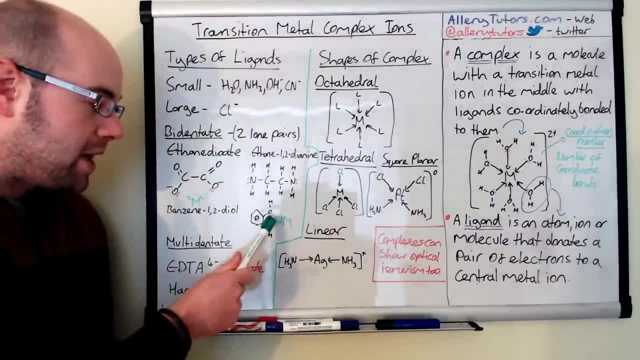 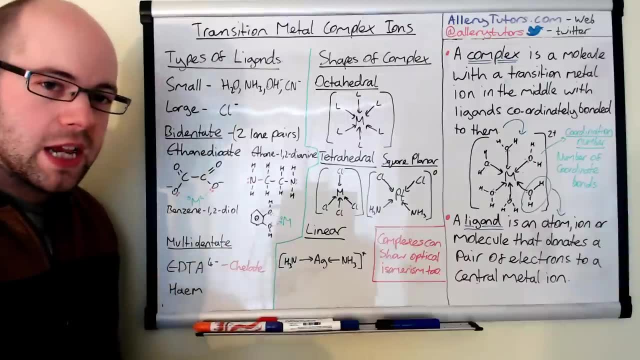 six times. So anything where we have more than two long pairs being able to be donated to the same metal ion, we call that multidentate, And one of the most important multidentate ligands is heme, And heme is found in obviously in your red blood cells and forms hemoglobin. 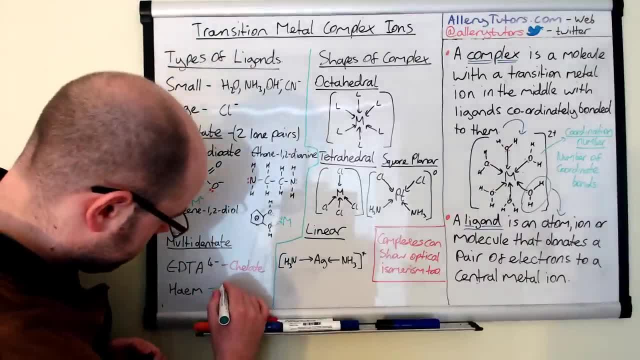 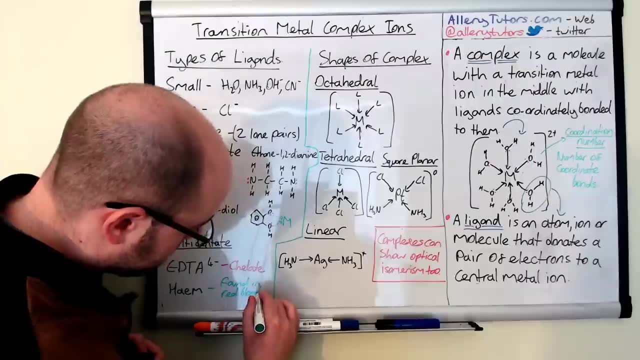 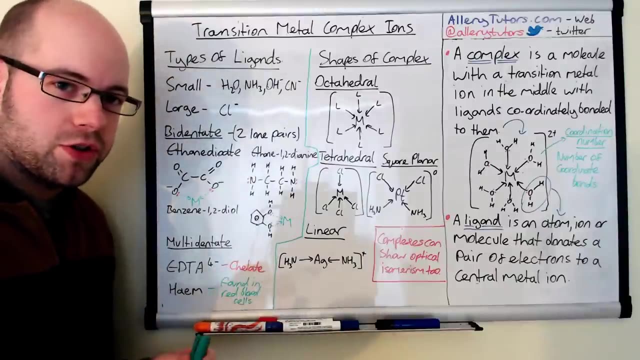 So this is found in red blood cells, So I'll put that on there: Found in red blood cells. And these are really, really important because actually this is responsible, or part of a hemoglobin is responsible- for carrying oxygen around the body. 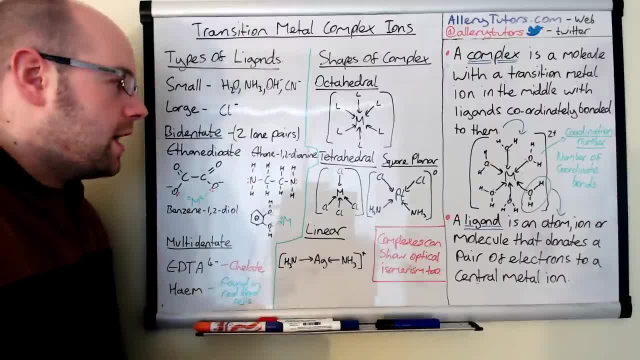 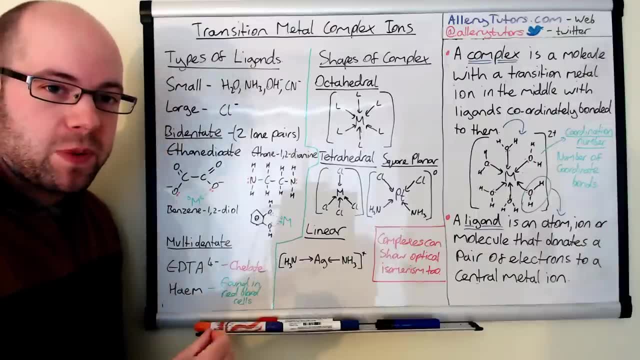 to allow it to, so cells can use it to effectively respire. So- and this is also important as well, because it explains why some ligands, for example cyanide, is really toxic, as it can displace oxygen within the hemoglobin. 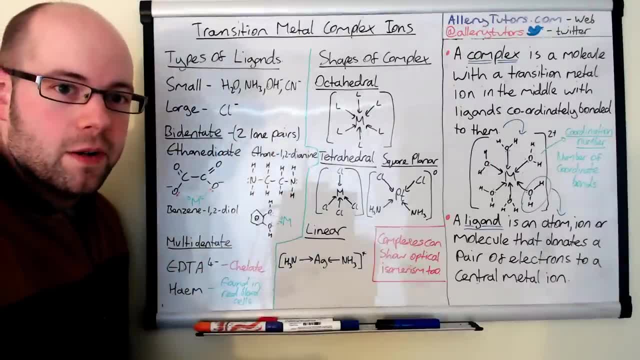 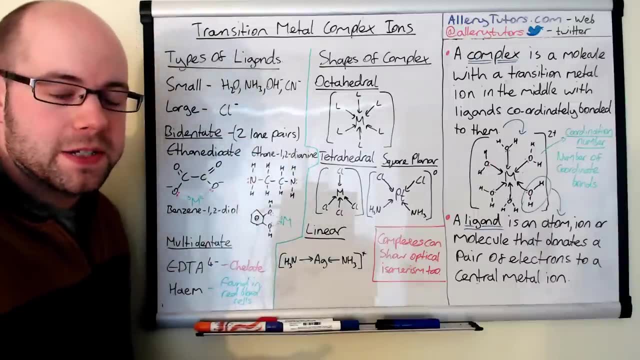 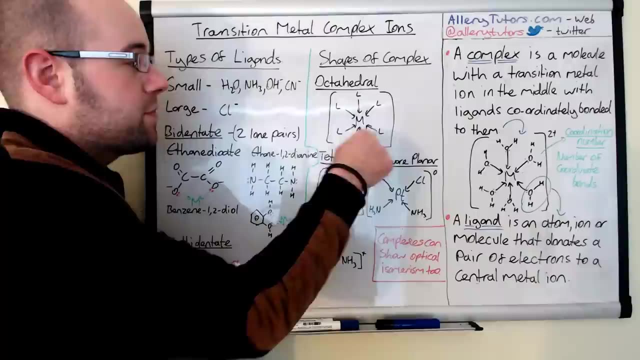 And instead cyanide is around there instead, And this can obviously reduce the oxygen content in the blood and can be lethal. and is lethal, And same with carbon monoxide has a similar effect as well. Okay, So just quickly looking at some of the shapes of these complexes as well. We have 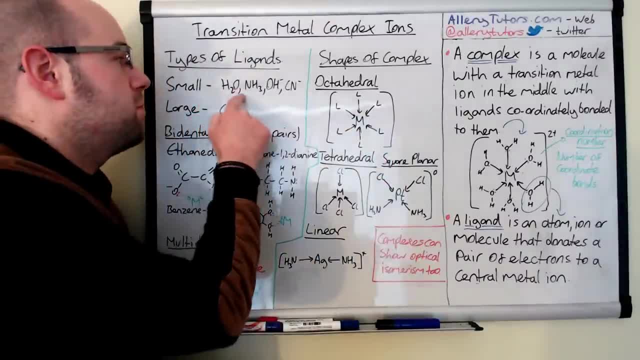 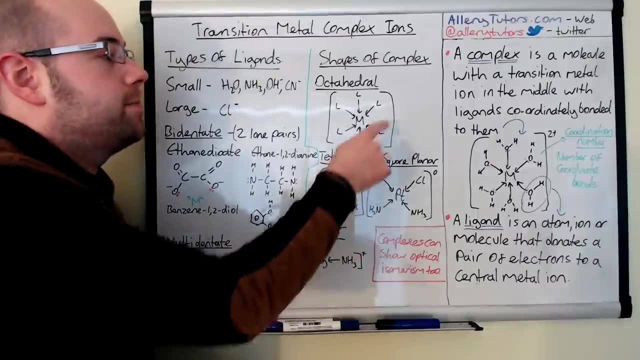 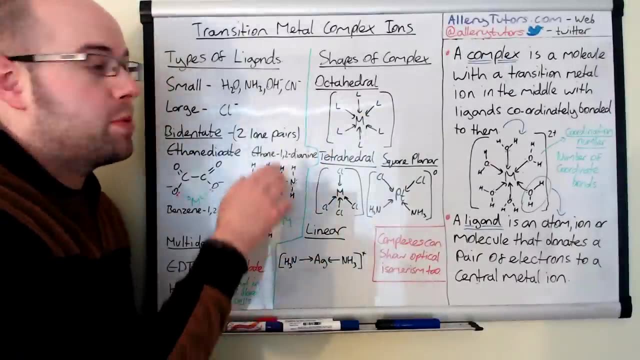 something called an octahedral shape. Now this is formed when we have small ligands like water, ammonia, hydroxide and cyanide. You can fit six of these around the metal ion and it forms an octahedral complex. Now it is worth noting the- I haven't put a charge up here, but these, if they have a charge. 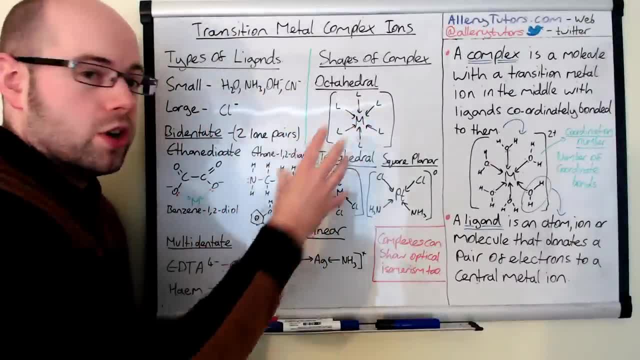 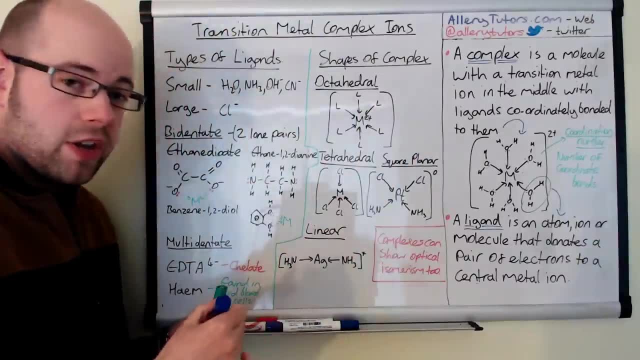 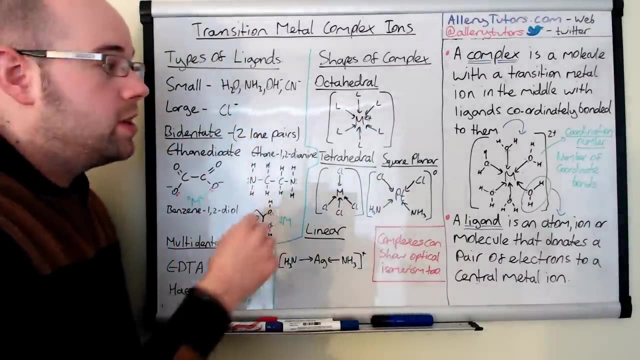 if the ligand itself has a charge, it will have an effect on the overall charge of the complex. So for example, if we have a- let's say, this metal ion in here is a two plus charge, then if we surround this complex with six waters, water is neutral so therefore has no charge and therefore the overall 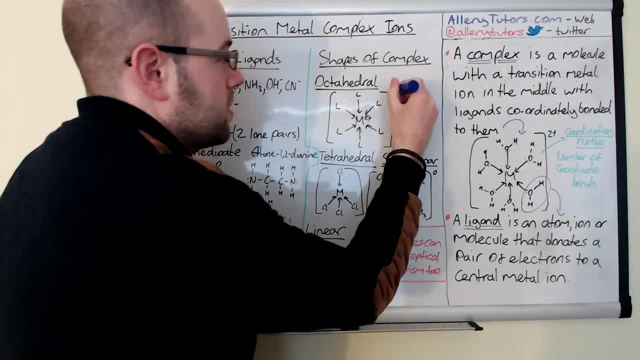 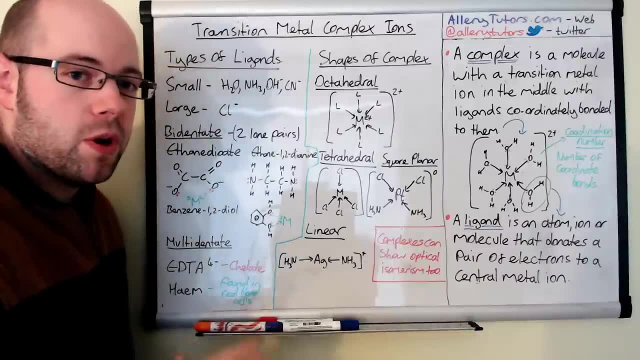 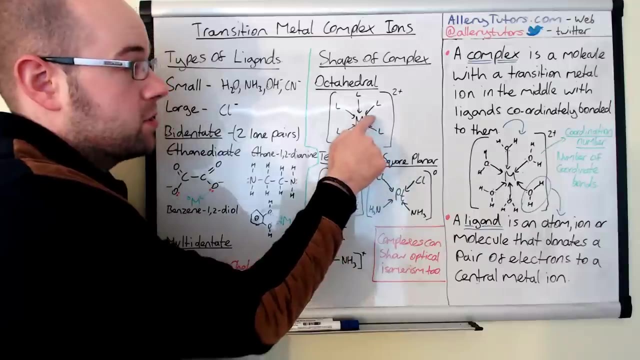 charge in the complex will be plus two or two plus, So we'll put that one there. if that was six waters surrounding it, Let's say two of these ligands were hydroxyl ions, so OH minus, and the rest were water. Effectively, the two OH minuses will cancel out the 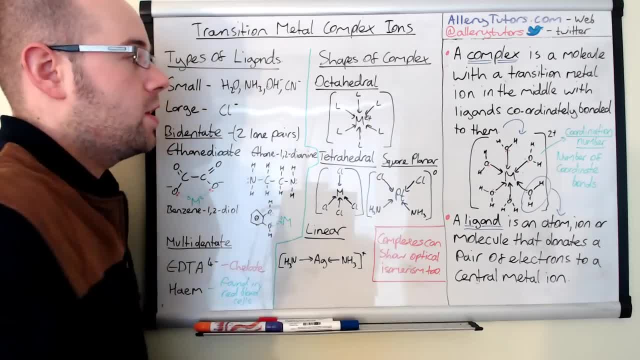 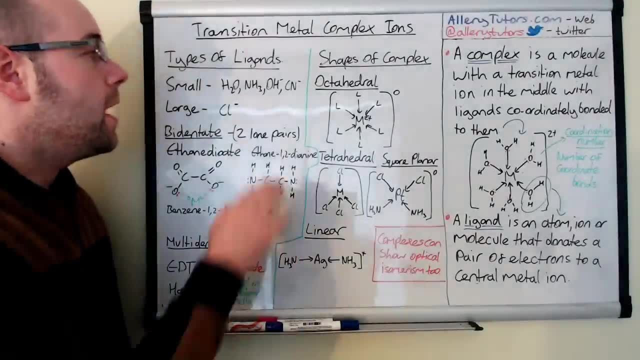 two plus charge in the middle and we would effectively have no charge on the top. And sometimes we can put zero on there to represent that the complex is actually neutral. And sometimes we can completely replace all of the ligands. So we have a two plus charge in the middle and all of the 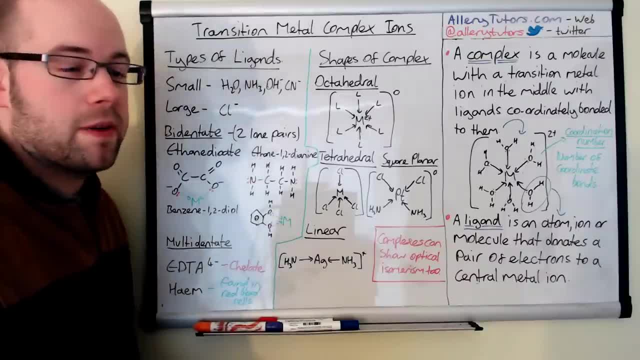 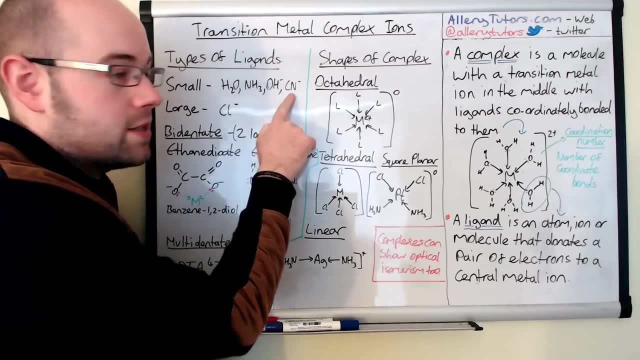 ligands are neutral, So we have no charge on the top And sometimes we can put zero on there. to say, for example, we might put six cyanide ligands around there. if this was a 2 plus charge in the middle and we swapped all these six water ligands for cyanide ligands, cyanide is minus one. 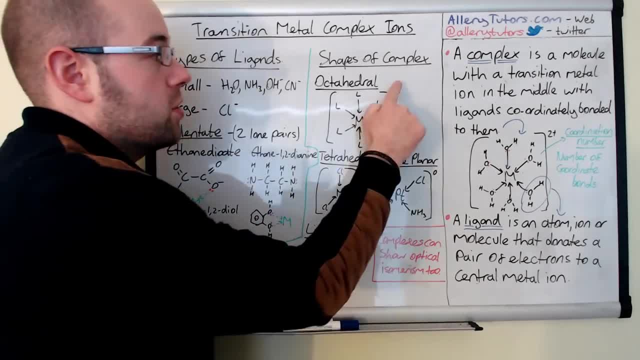 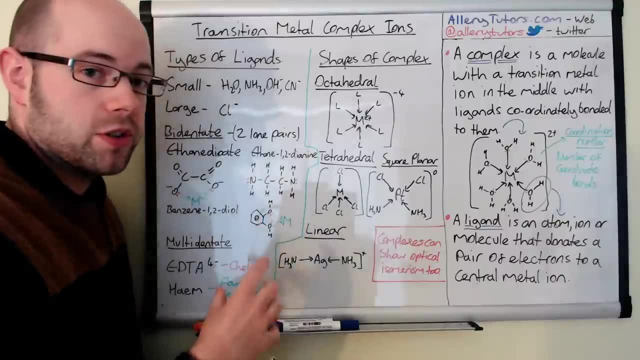 if we have six of them surrounding there, the overall charge left behind would be minus four or four minus, and that would be the overall charge on the complex. So it is important to take into account the charges of the ligands, as this will have an effect on the overall charge. 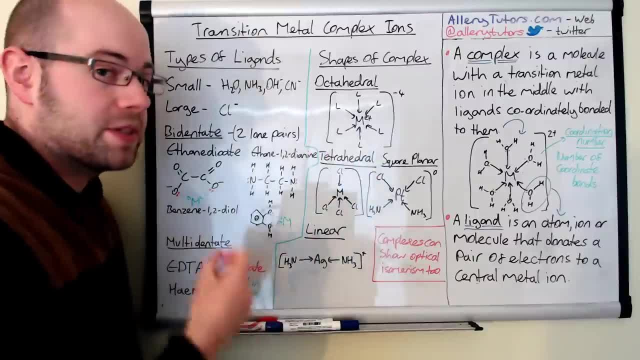 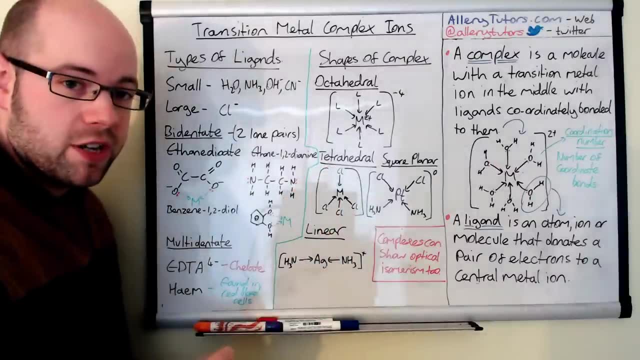 of your complex as well, and you don't just have to have six of the same ligands, you can have different ligands as well surrounding that Meth line. Okay, so just come around to the other one, tetrahedral. normally this is formed by larger ligands, such as chloride, and you can see here: 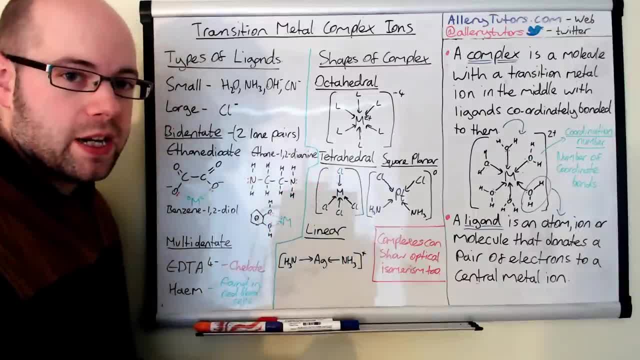 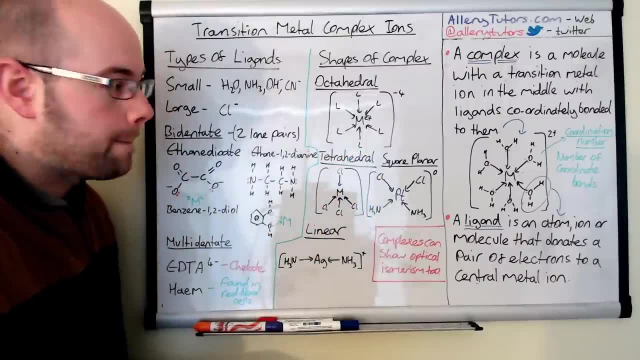 that we have four chlorines here. it's a much bigger ligand. we can't fit as many chlorine ligands, can't fit six, sorry- around the Meth line in the middle, so we just have to settle for four. Okay, sometimes we can have square planar. 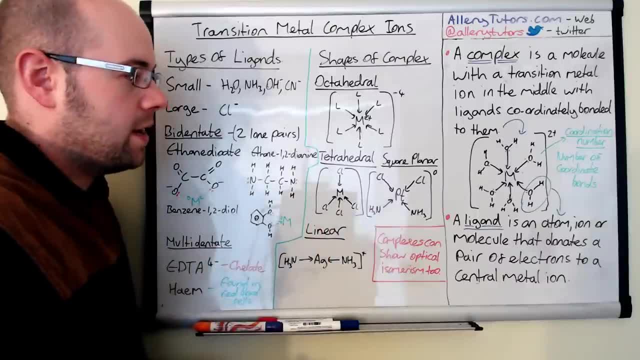 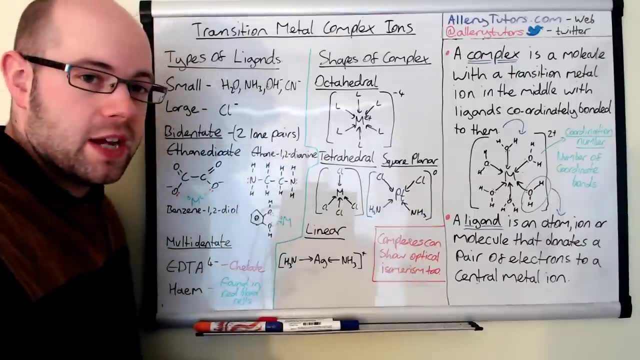 or square planar or square planar. Sometimes we can have square plane molecules as well. The specific example is something called cisplatin, and this is an example here. It's an anti-cancer drug and it can bind to DNA and stop cancerous cells from. 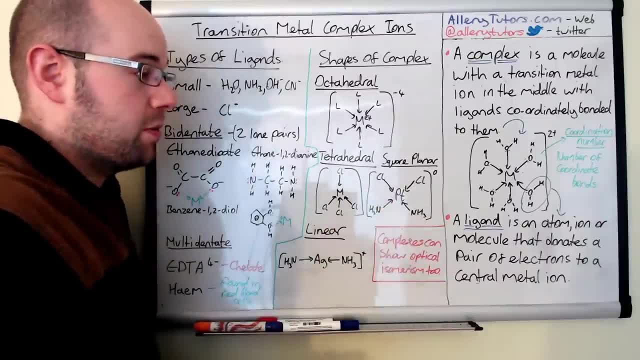 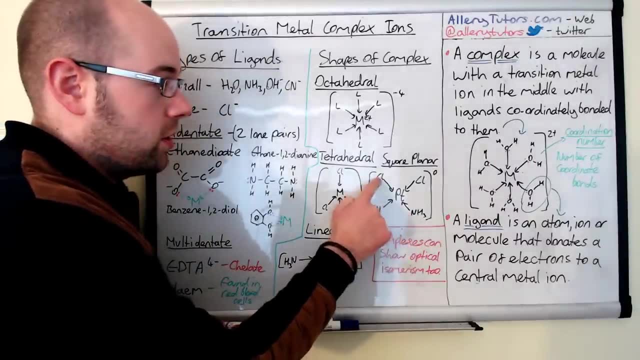 replicating, and so it's really useful. and this is the actual formula for cisplatin. Notice it doesn't have an overall charge and hence, because we know that ammonia is neutral and chlorines are minus one each, we must know that the platinum must have an oxidation state of plus two by just 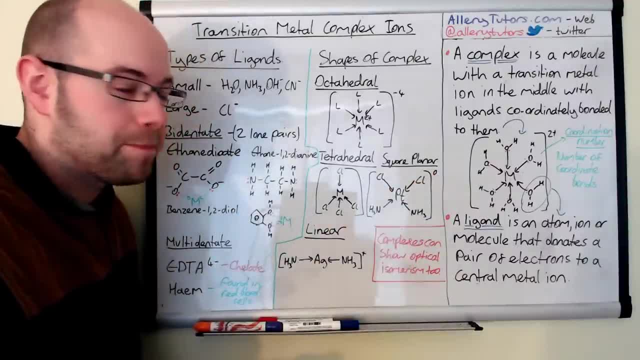 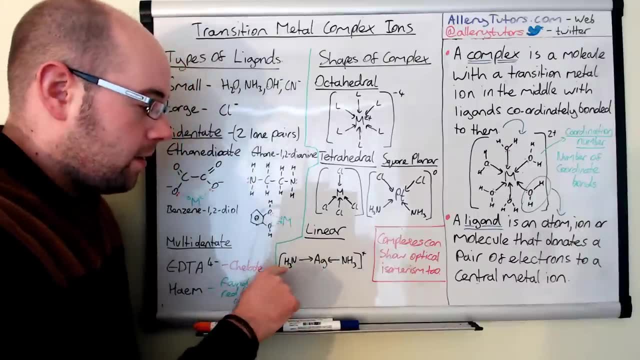 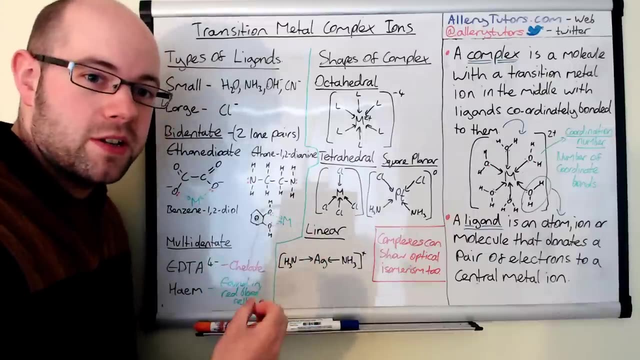 looking at the overall charge on there so you can work out backwards as well. Okay, just look at the last one here, which is linear. Again, linear ones have 180 degrees across the, across the silver layer. This is an example of Tollens reagent and you might use this for. 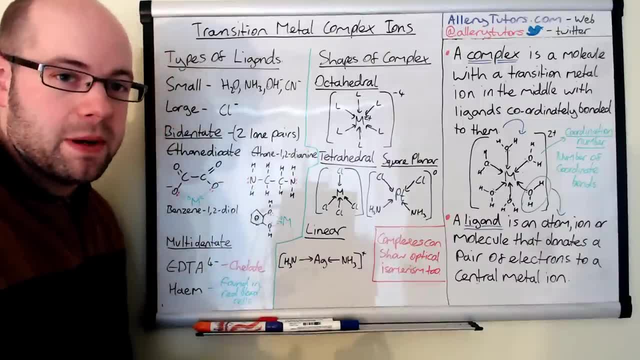 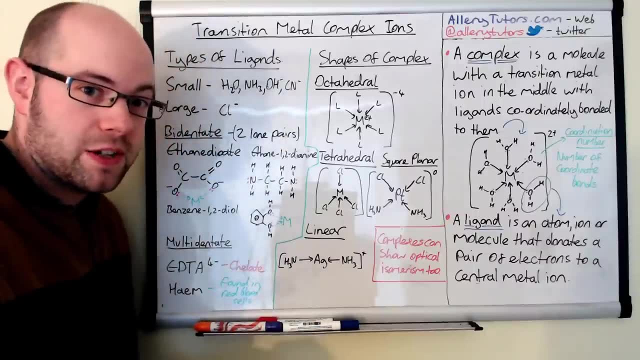 detecting aldehydes and it will give the silver mirror and this is the reagent that we would use. And if you're doing some example, don't you want this and some don't, so it's best to check the specification to make sure you know if this, if you need to know that, one Again, another one as